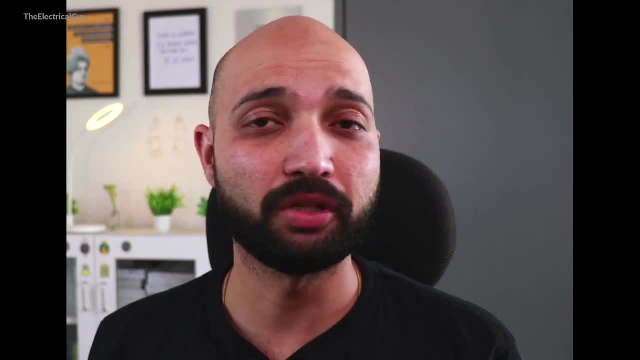 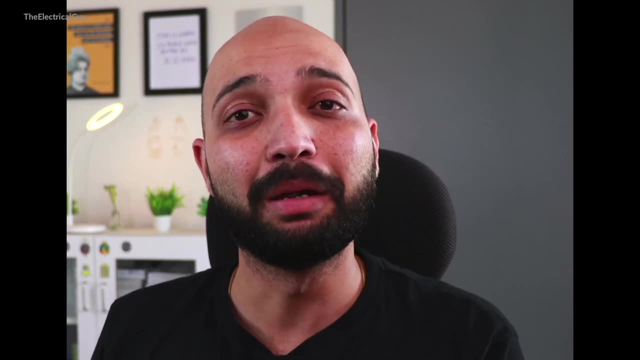 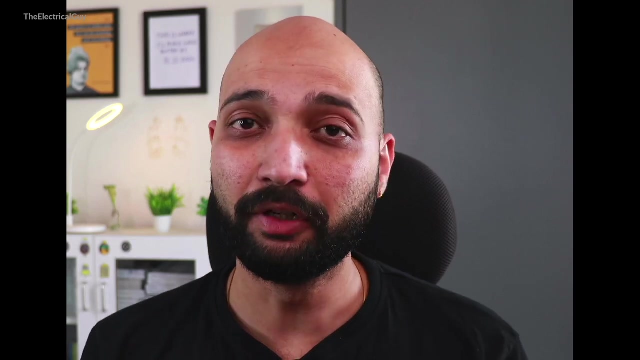 If you are into AC circuit calculation, then understanding the term impedance is of a key importance and as you progress your study in electrical engineering, the term impedance get more and more important, because we are going to deal a lot with AC circuits and this video is going to help you out to understand the term impedance in easiest way possible. So if you 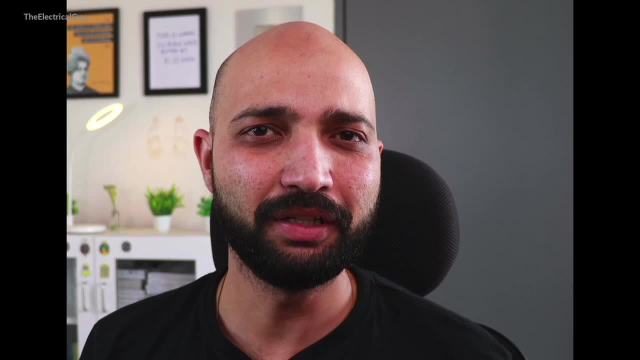 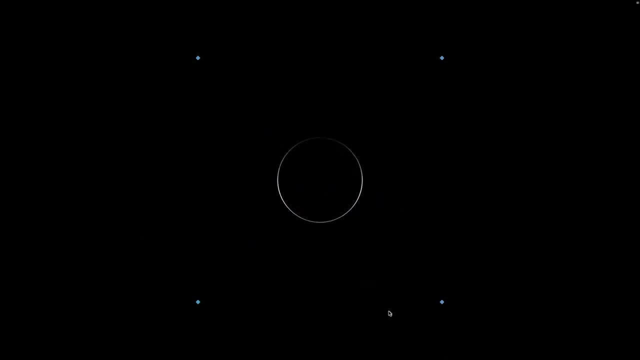 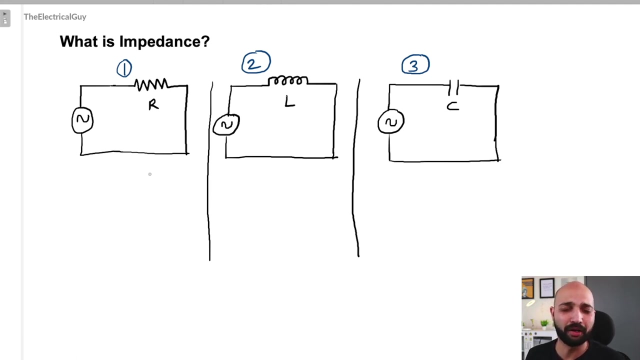 want to get all these details, you need to watch the video. And before we start, if you are new here, my name is Gaurav J. I post videos related to electrical engineering on this channel in the easiest way possible. So if you are interested in learning, 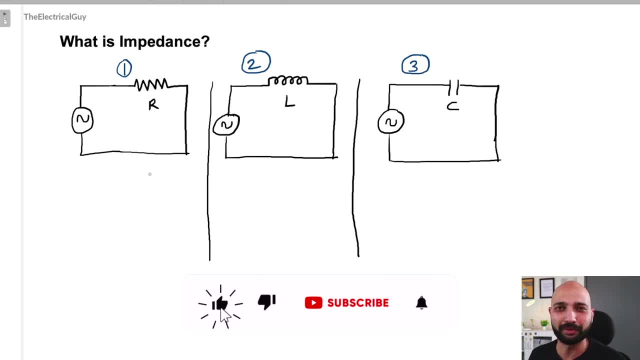 electrical engineering in easiest way. make sure you subscribe to this channel and click on the notification bell icon so that you get notified every time I upload a new video. Now let us start with what is impedance Now? the first circuit that you can see on your left hand side consists of a AC source and a 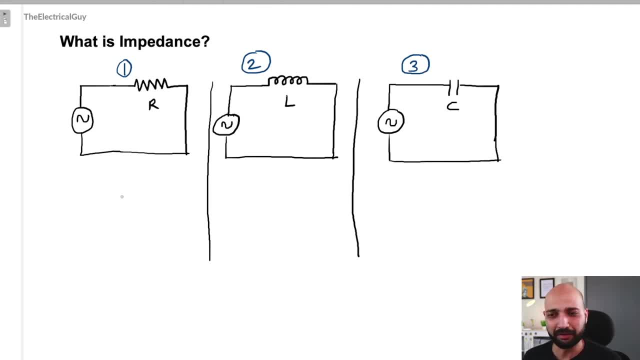 resistor. So we can call this circuit as purely a resistive circuit and, as a result, this circuit is only going to offer a resistance to the flow of electrons. Now moving on to the circuit 2.. Now this circuit consists of a AC source and an inductor. Now this we can call as purely inductive. 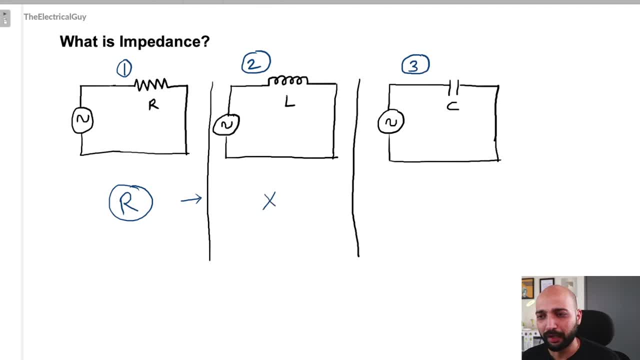 circuit and, as a result, it is going to offer a resistance to the flow of electrons. So we can only offer reactance Now. since this is specifically offered by an inductor, we call it as inductive reactance XL And, by the way, it is important that you understand these terms. what is inductive? 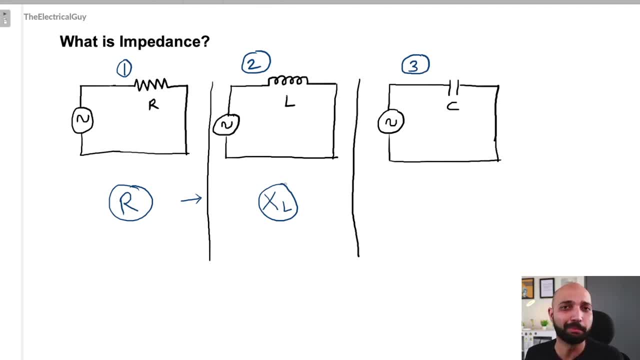 reactance. what is capacitive reactance? to understand the term impedance: If you don't know what are these terms, then I have a dedicated video on inductive and capacitive reactance. I'll provide link for that down in the description. You can go and check that out. So the circuit number 2 is going. 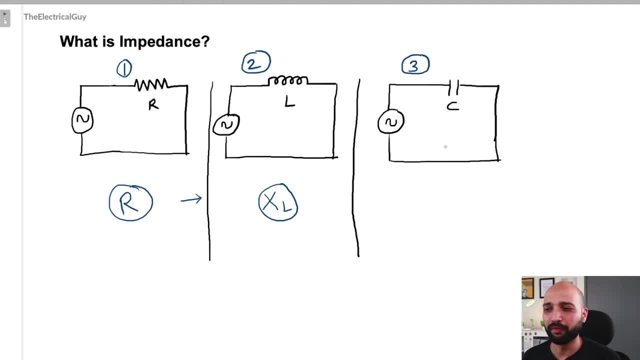 to offer inductive reactance to the flow of electrons. Now, moving to the third circuit, is it has a AC source and a capacitor connected, So we can call it as purely capacitive circuit. So what this circuit is going to offer? it is going to offer a reactance, but since it is offered by a capacitor, 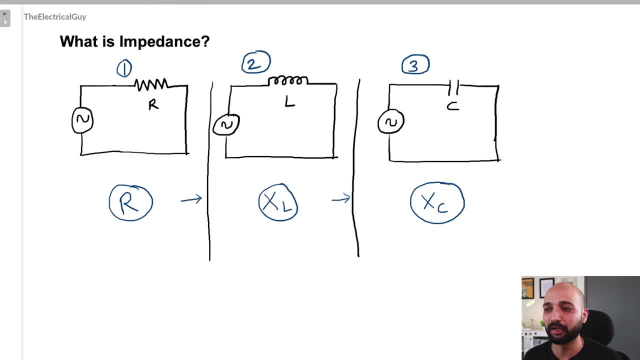 we call it as capacitive reactance. So this circuit is going to offer capacitive reactance. So if you want to understand the terms of this circuit in detail, then you need to know that these terms are ideal and these are perfect, So definitely they don't exist in the practical world. Resistive- 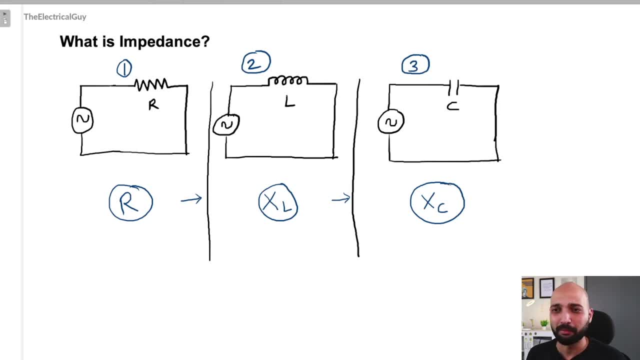 circuit only offers resistance, inductive circuit only offers inductive reactance and capacitive only offers capacitive reactance. But if we talk about the practical world, this situation you will not find. You will always find combination of different, different opposition that is being offered in a circuit. 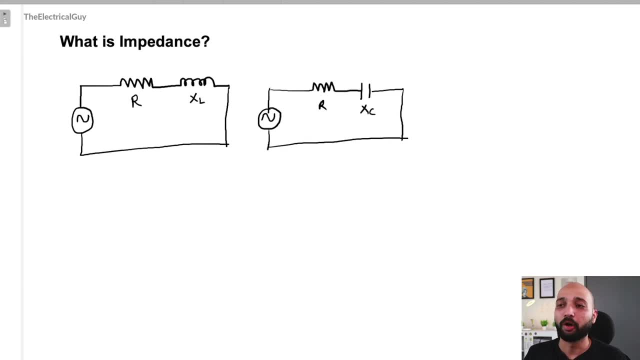 So, for example- and it also has an inductor- or there can be situation where resistor is there, or and capacitance is there, or there will be a situation where the circuit can experience all the three oppositions, right? so, taking the example of the most relevant case in the practical, which is the combination of resistance, inductance, 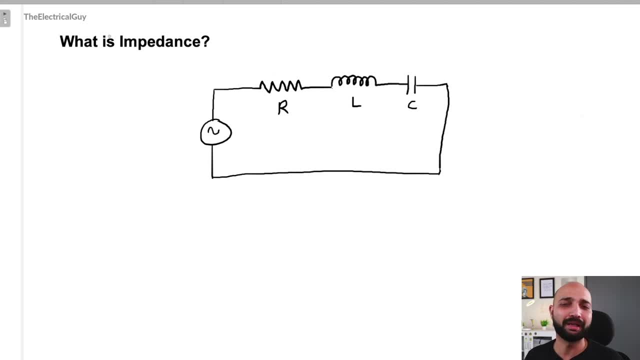 and capacitance. this is the most common practical circuit arrangement. you will find it the combination of all the types of opposition. so now, talking about this circuit here, the flow of electron or the AC will not be only getting resistance right. there are inductor, there are capacitors in the circuit, so definitely. 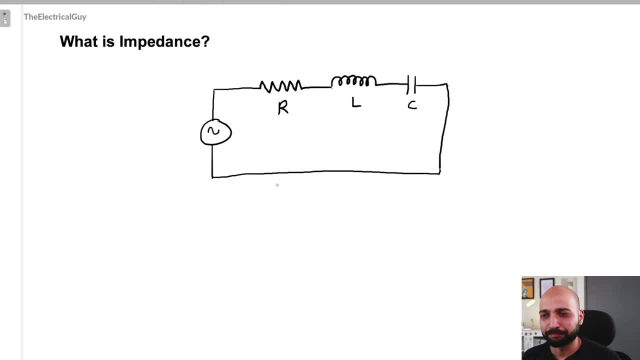 they will also be offering some opposition. so the resistor here, this will offer a resistance clear plus. we also have an inductor here, so it will offer inductive reactance plus. we also have a capacitor here, so it will also have a capacitor here, so it will also have an. 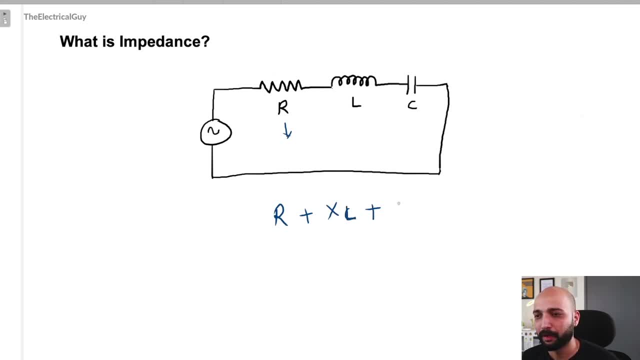 capacitor here, so it will also have a capacitor here, so it will also have a capacitor. sorry, this is X L and the capacitor will offer X C, so this circuit is experiencing all this position. now you cannot say the circuit is resistive, or you cannot say the circuit is. 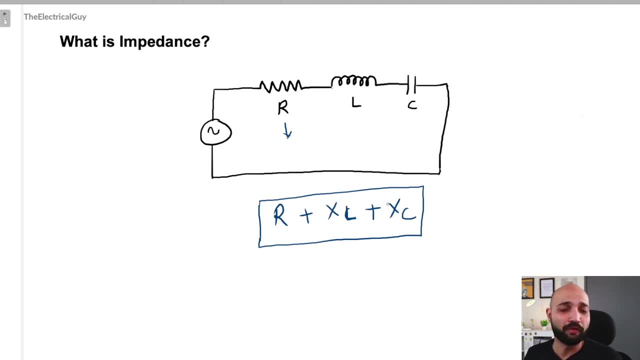 reactive, it is combination of all the opposition. so definitely we need a term which is more comprehensive, which is more broader and which can cover all these three opposition, and hence we have a dedicated name for this opposition and we call it as impedance, The combination of all the types. 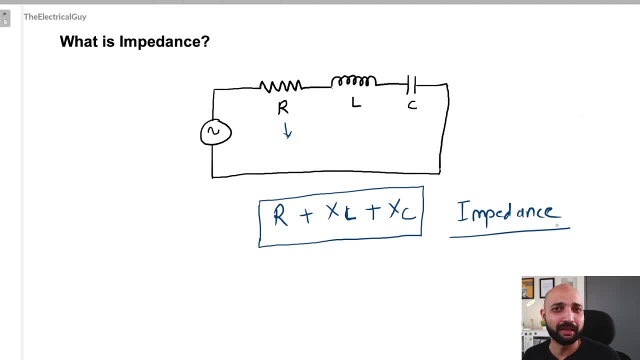 of opposition is what we call as impedance. Now, just like resistance or reactance, it is also measured in ohms and it is denoted by letter Z. So if you have to find out the opposition that this circuit is offering, you just have to add all these oppositions together and 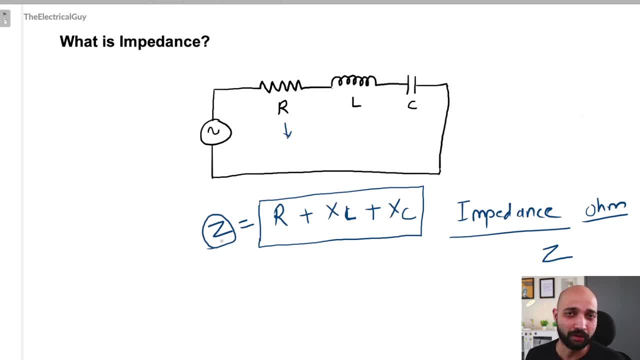 then you will get an impedance. So understood what is impedance and with the help of this impedance we can also make a ohms law for AC circuit and we can say: voltage is equals to current times, the impedance. So this, you can refer it as ohms law for AC circuit. and 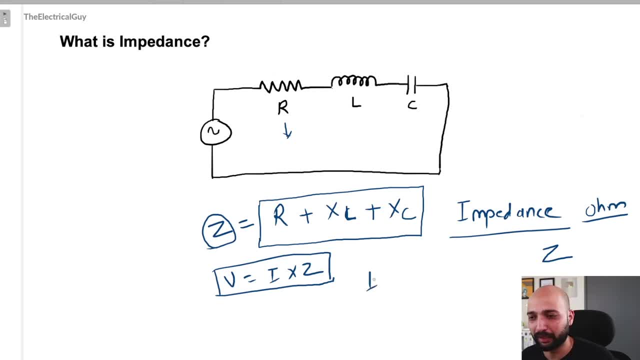 with the help of this ohms law, you can identify different parameters like current. So I is equals to voltage divided by impedance. or you can also find out the impedance of the circuit, or impedance is equals to voltage divided by current. So understood, this is the impedance. Now, if you want to write the term definition for impedance in proper way, 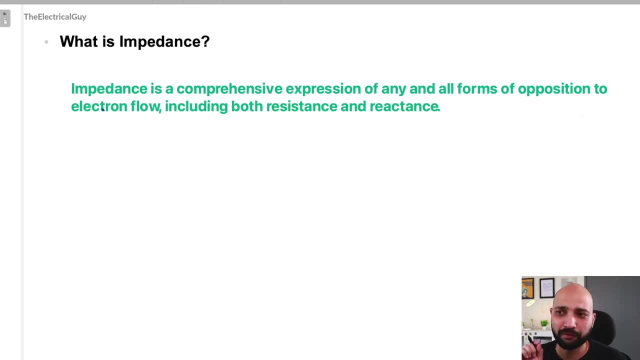 then you can write: impedance is a comprehensive expression of any and all forms of opposition to electron flow, including both resistance and reactance. Now this is a really important sentence here: that impedance is a comprehensive expression. So even if your resistance, you can call it as impedance in AC circuit. Now we are talking. 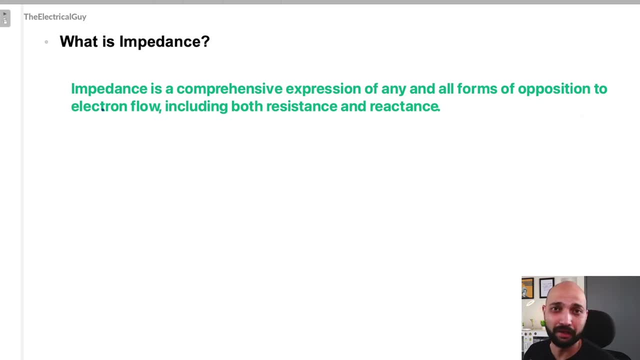 about AC circuit. the impedance term is not applicable in case of DC. So even if your AC circuit is having only resistance, you can refer it as impedance, and that makes more sense. or if your circuit only has reactance, you can refer it as impedance in case of AC. 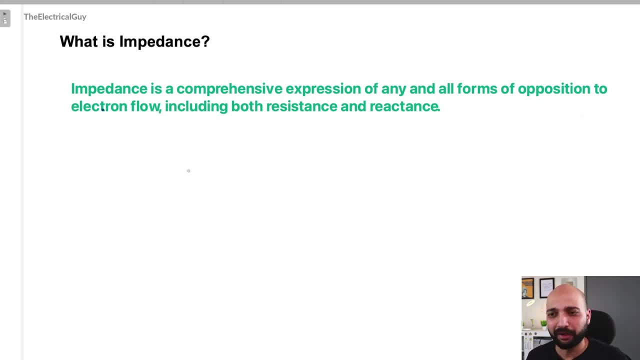 circuit. Now let's talk about a perfect resistance, for example. Now perfect resistance is consists of: it will offer 100% resistance. So let's say 100%, 100 ohms it is offering and the resistance will not have any sort of reactance in it. We are talking about perfect resistance. So 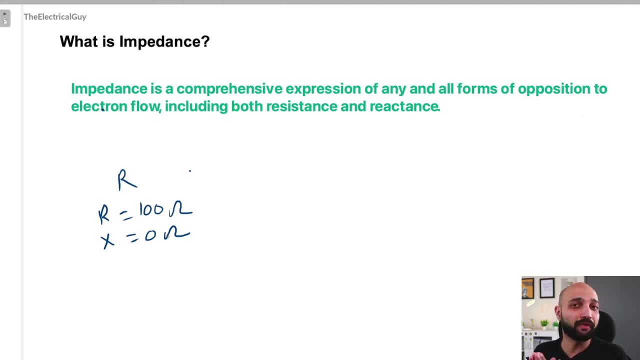 it will only offer resistance. it will not have any sort of reactance, right, and you can also refer it as impedance. So impedance will also be 100 ohms, right, clear. Similarly, when we talk about reactance or let's say inductor here, inductor, a perfect inductor, will not have any resistance to 0 ohm, it will. 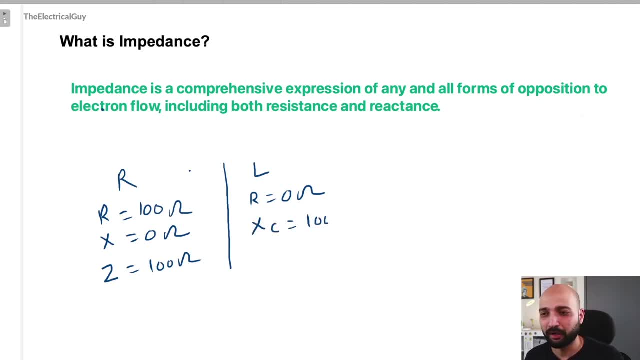 only offer inductive reactance, let's say 100 ohms. and since in case of inductive circuit, voltage and current are out of phase by 90 degree, we write angle as 90 degree. It shows the angle between voltage and current. So in case of inductive circuit the voltage is 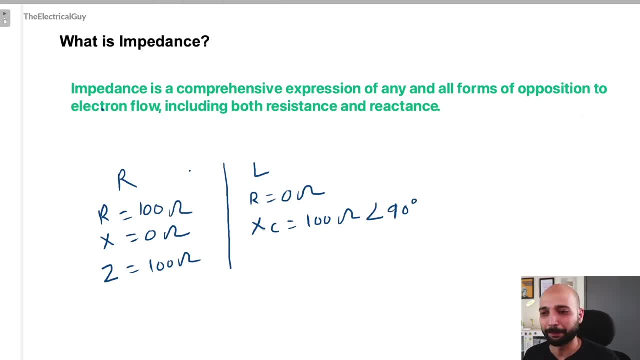 leading current by 90 degree, and hence it is 90 degree, and you can also refer this as impedance is 100 ohms and the angle is 90 degree. Similarly for capacitive circuit, again, a perfect capacitor will not have any resistance to 0 ohms. it will have XE. sorry, this is XL. 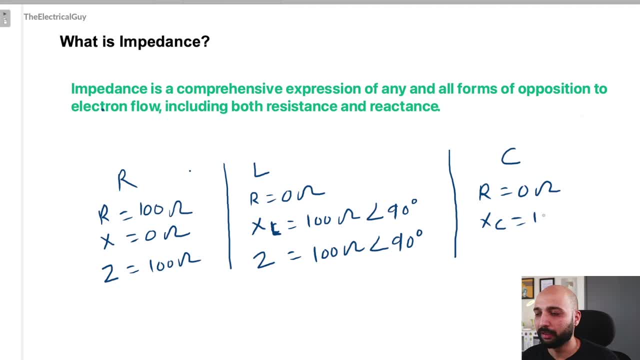 here, Not XE. So XE will be, let's say, 100 ohms, but the angle between the voltage and current will be negative 90 degree. and why is that? because in case of capacitive circuit, voltage lags behind the current by 90 degree, and that is the reason why it is negative 90 degree. 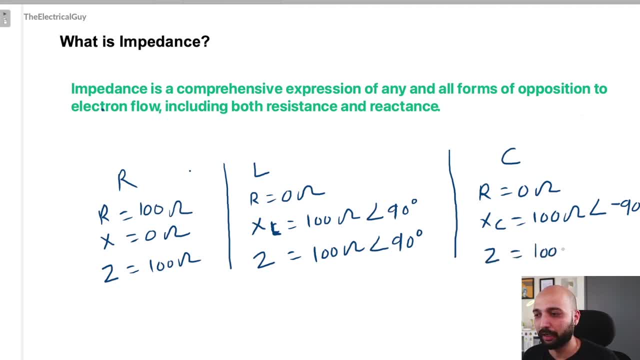 So you can also refer this- as impedance is equals to 100 ohms and the angle is negative, 90 degree, right. So impedance is really important To understand in order to understand the AC circuit, and it is a comprehensive term which we can use for all the types of opposition that is being offered to flow of electron. 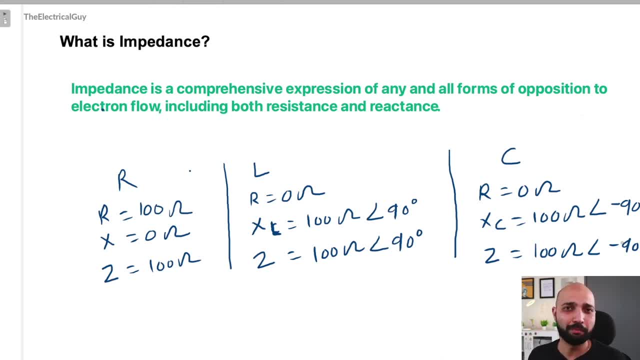 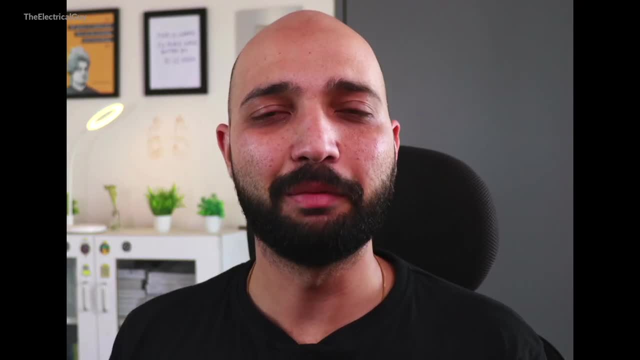 in AC circuit, So understood the concept of impedance. it is really really easy to understand and also equally important. So I hope this video has helped you in understanding something important today and if it did, please do like the video and click on the subscribe button. that really helps the channel to grow. 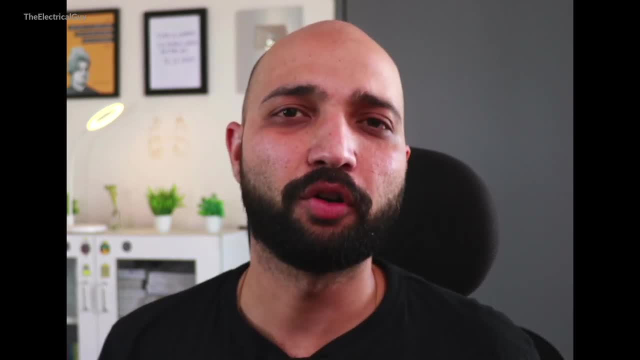 further and I really, really appreciate that. So thank you for watching. I will see you in my next one, but till then, keep watching, keep learning.